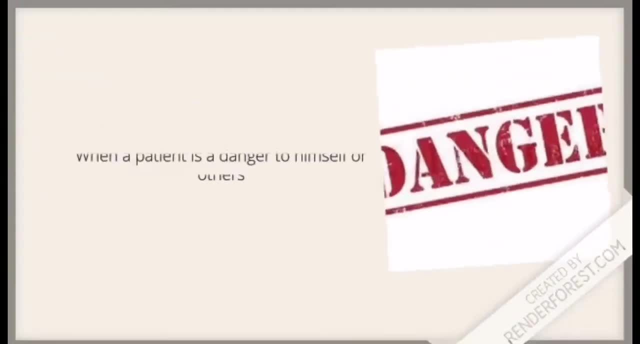 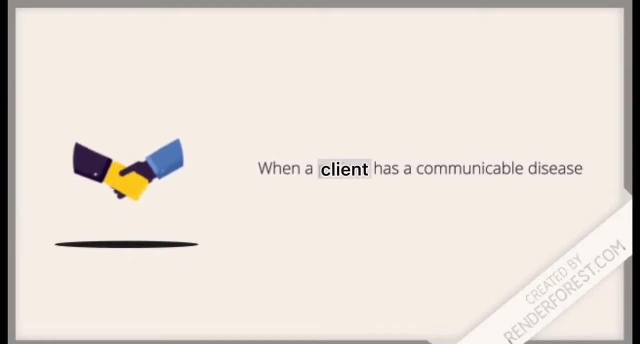 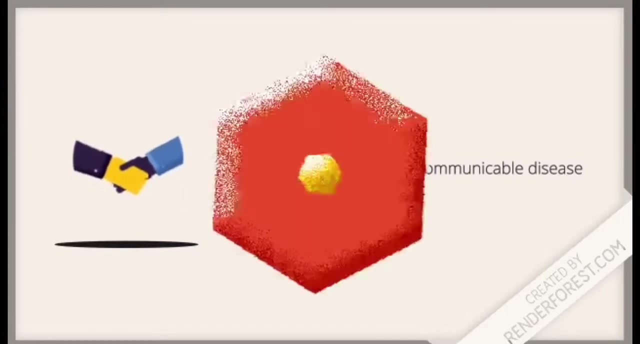 Confidentiality can be broken when a client is a danger to himself or other. Second, when a client has a communicable disease, such as, process must be followed and ethical justification of the prevention of harm to other must be clear. Lastly, when a client gives consent, 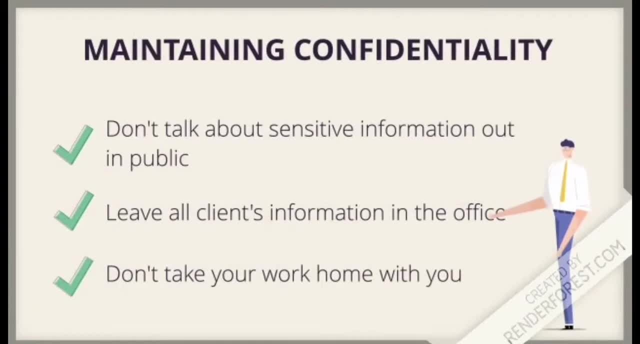 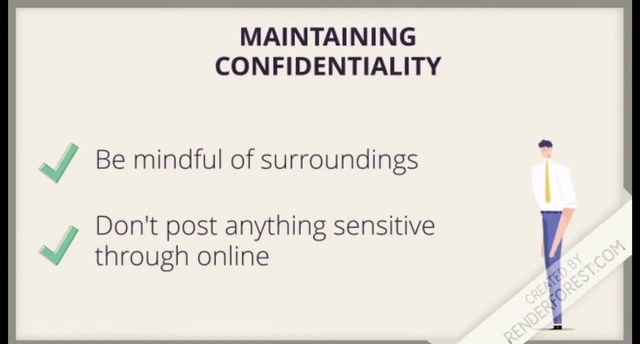 Next points is maintaining confidentiality. First, don't talk about sensitive information out in public. Take the conversation elsewhere, if need be. Second, leave all clients' information in the office. Third, don't take your work home with you. It's means not talking about work matters to friends or family. 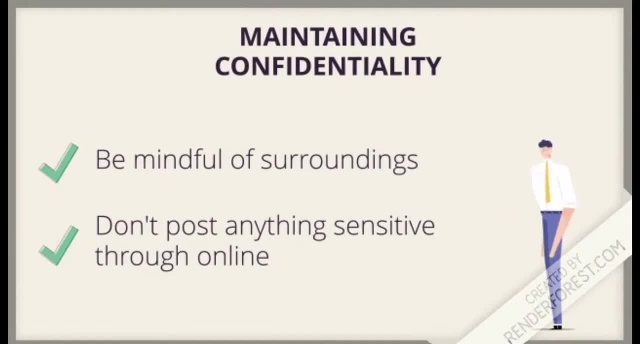 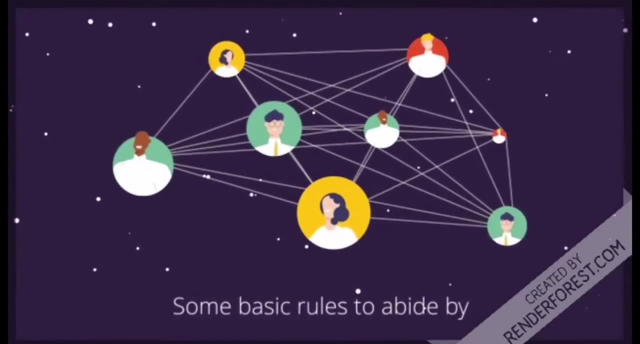 Fourth, be mindful of surroundings. When you are on the phone, people couldn't be listening. Fifth, don't post anything sensitive online from general tips. workplace Confidentiality plays a big role within your company and personal safety company. let's look at some basic rules to abide by: secure important files, whether this is digital. 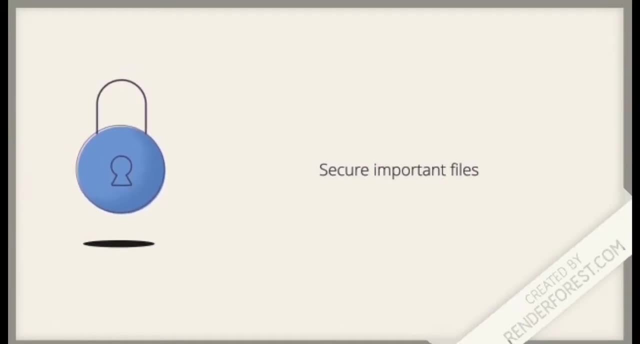 or paperwork. client information should always be kept in a secured cabinet or folder. encrypt your files. it's very important that you send emails through an encrypted channel or network using connection or a company provides encryption software. lastly, proper organization: always label your files and folders accordingly so you can stay aware of those that are confidentiality. 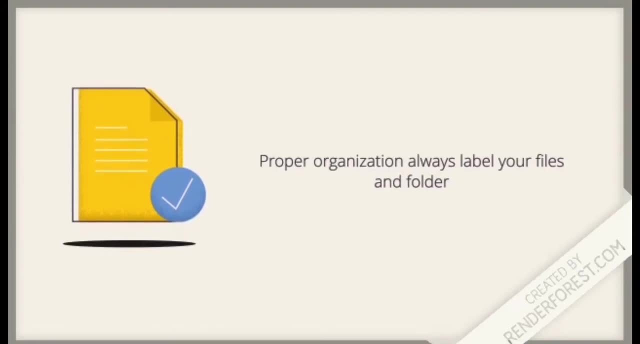 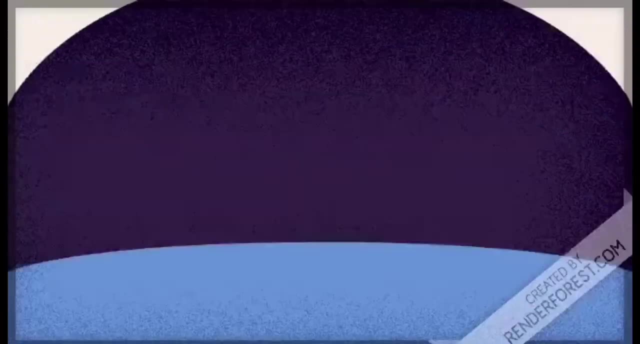 those that are not. it is good practice and it's helped to remind us how easy we could leak.